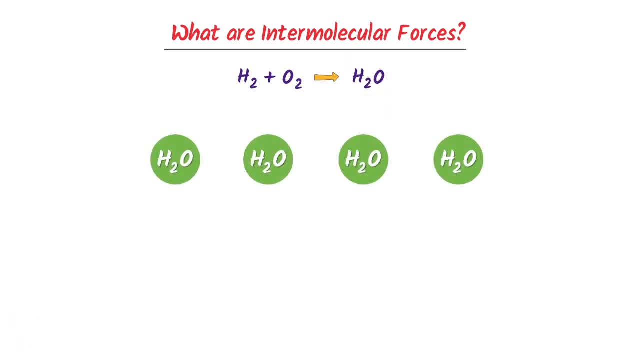 oxygen. Now consider these four molecules of water, or I say four basic units of water. Let me ask you what are holding together these four molecules of water, or these four basic units of water? Well, there is attractive force between these two molecules of water. there is attractive. 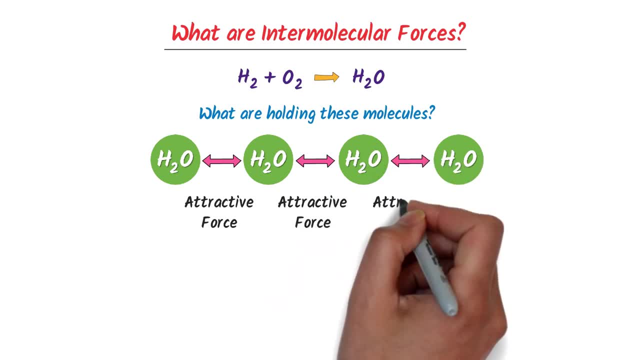 force between these two molecules of water, and there is also attractive force between these two molecules of water. So the answer is simple: Attractive forces are holding together these four molecules of water. In chemistry, these are the two molecules of water. In chemistry, these are the two molecules of water. 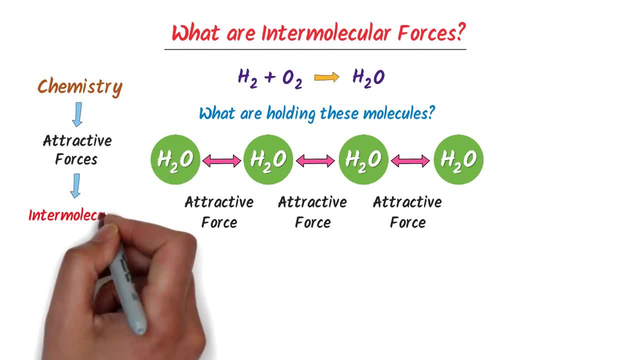 Attractive forces between molecules are called intermolecular forces. Let me repeat it: In chemistry these attractive forces between molecules are called intermolecular forces. Thus we say that intermolecular forces exist between these two molecules of water. Intermolecular forces exist. 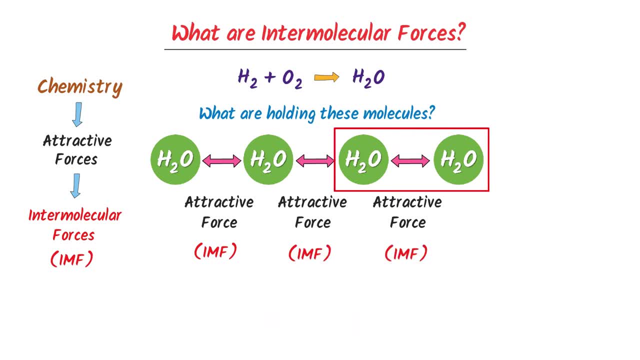 between these two molecules of water, and intermolecular forces also exist between these two molecules of water. Intermolecular forces exist between these two molecules of water and these two molecules of water. Therefore, we define intermolecular forces as the attractive or repulsive. 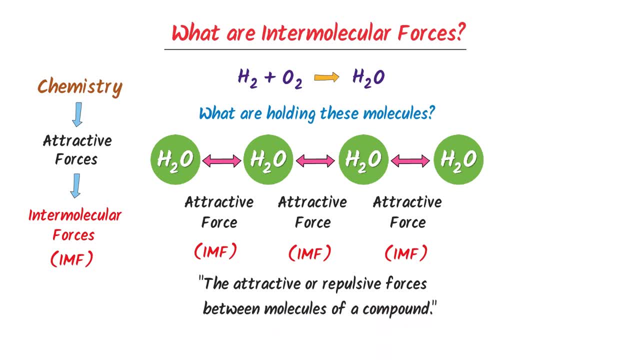 forces between molecules of a compound are called intermolecular forces. Let me repeat it: The attractive or repulsive forces between molecules of a compound are called intermolecular forces. Remember that intermolecular forces usually exist between molecules, not between atoms. 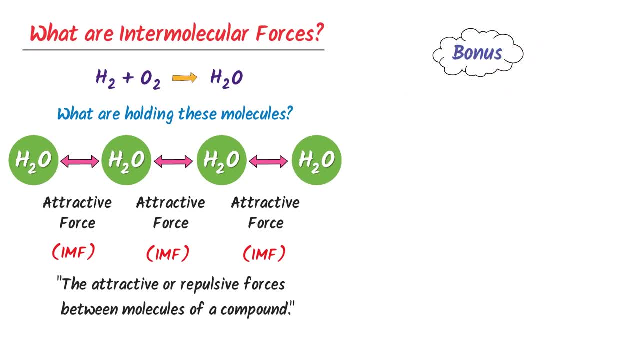 Here. let me teach you one bonus point. All intermolecular forces are electrostatic in nature. Consider case no.1 and case no.2.. In case no.1, this negative side of this molecule and this positive side of this molecule attract. 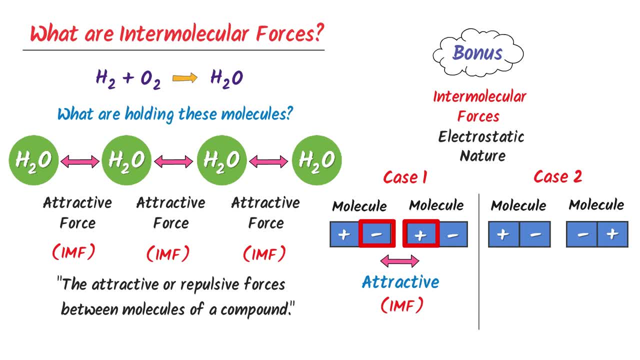 each other. so we say that here intermolecular forces are attractive, While in second case this negative side of this molecule and this negative side of this molecule repel each other. So we say that here repulsive intermolecular forces exist. 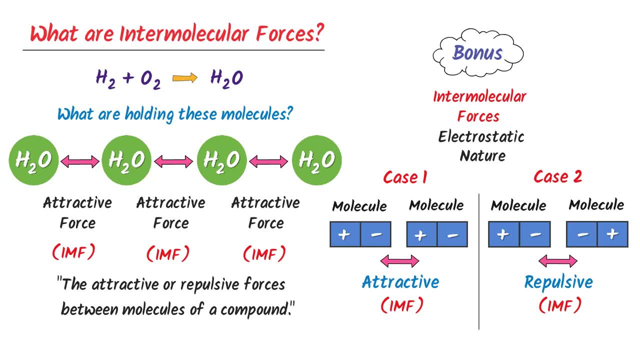 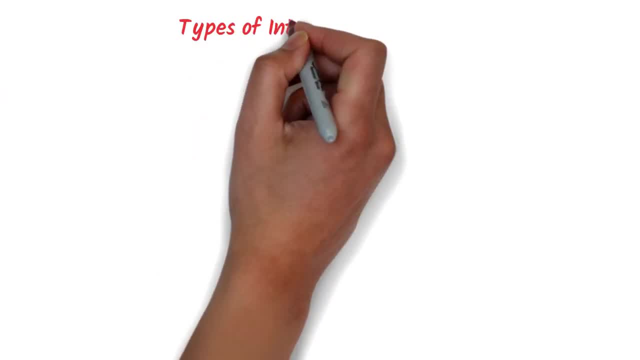 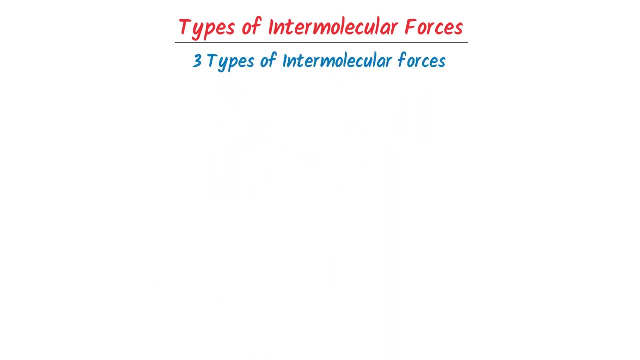 Therefore we say that all intermolecular forces are electrostatic in nature. Thus noted down this important point, Now let me teach you the different types of intermolecular forces. At college level, We only study three types of intermolecular forces, like hydrogen, bonding, dipole-dipole. 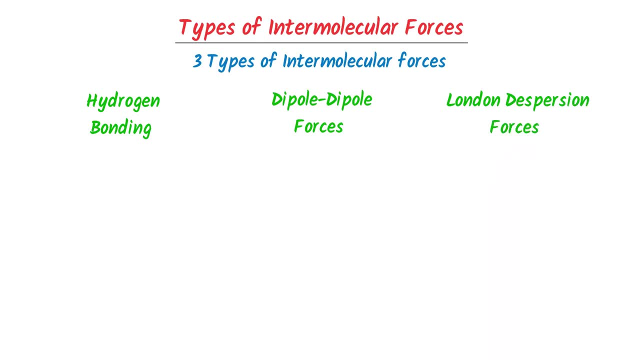 forces and London dispersion forces. Hydrogen bonding exists between molecules like water, hydrogen fluoride and ammonia. Dipole-dipole forces exist between two polar molecules like HCl, sulfur dioxide, etc. While London dispersion forces exist between two non-polar molecules like hydrogen gas. 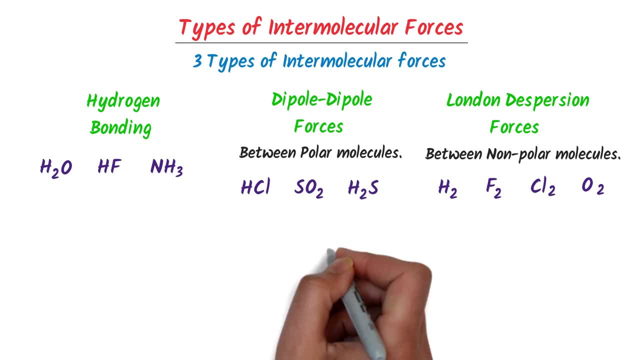 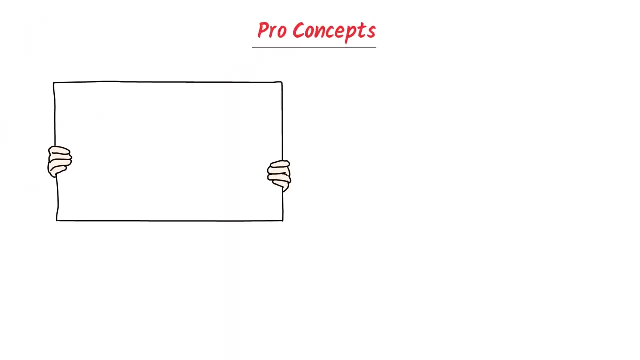 fluorine gas, chlorine gas, oxygen gas. If you want to learn more about these types of intermolecular forces, then watch our lectures, and their links are given in the description. Now let me teach you some concepts about intermolecular forces. 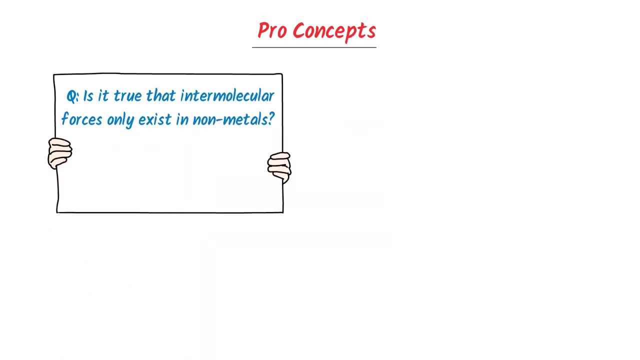 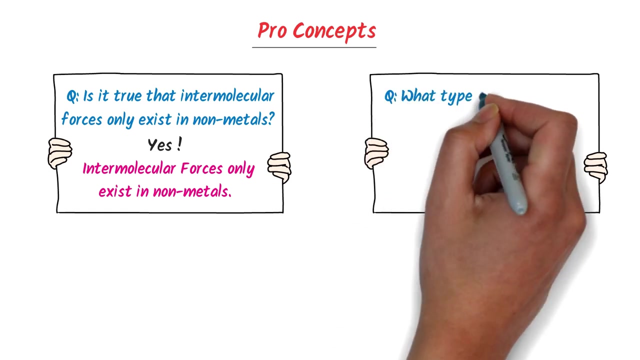 Is it true that intermolecular forces only exist in non-metals? The answer is yes. Intermolecular forces only exist in non-metals, while intermolecular forces do not exist in metals. Secondly, what type of intermolecular forces are present in metals? 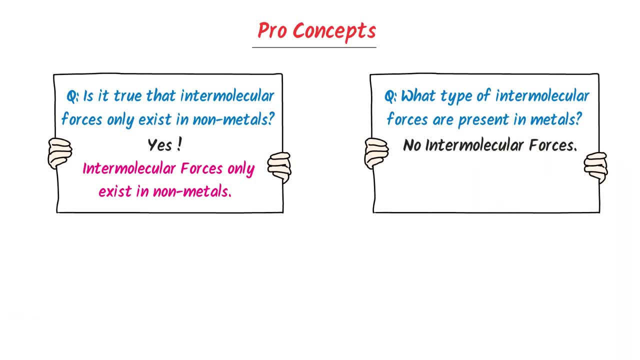 Well, metal contains no intermolecular forces. Rather, metal contains intramolecular forces, a chemical bond like metallic bond. If you want to learn more about intermolecular forces, then watch our lectures, and their links are given in the description. 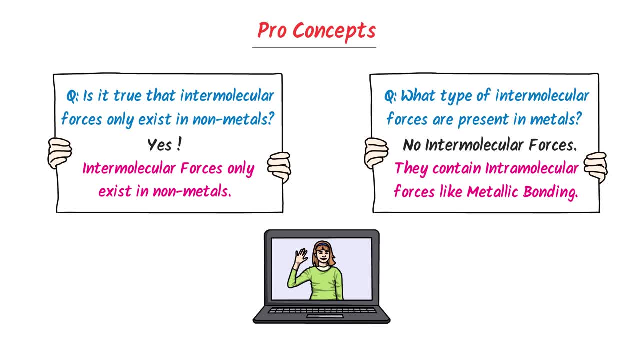 You must not forget to subscribe to our channel, like and comment on our videos, And if you read our books, you will also learn about intermolecular forces. If you want to learn more about intermolecular forces and intramolecular forces, then watch. 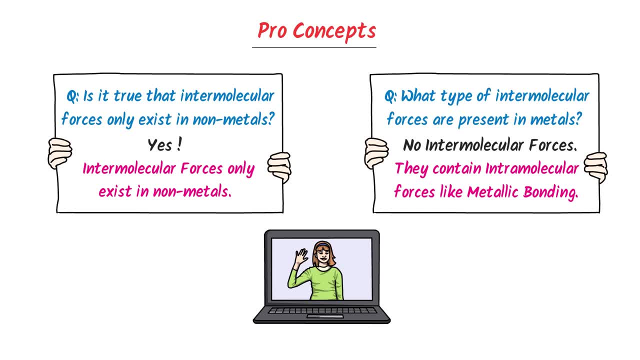 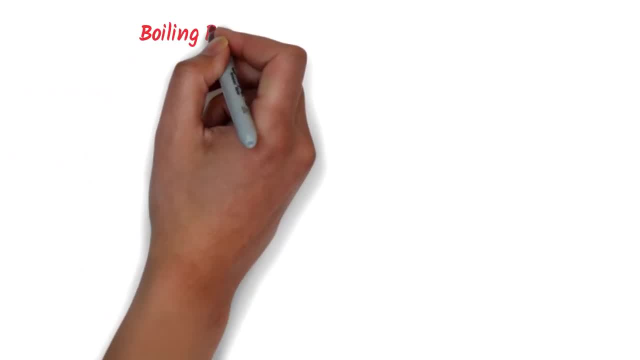 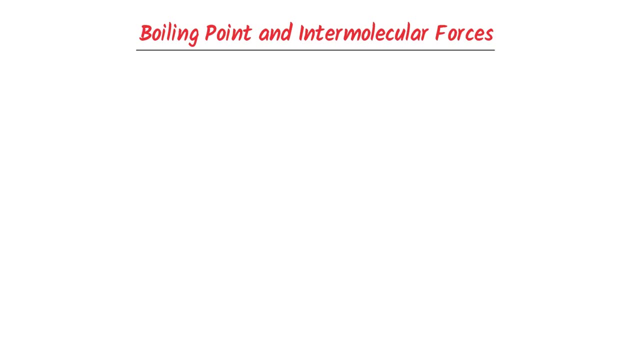 our lecture and its link is given in the description. Thus noted down these important questions. Also, you should learn that what is the relationship between boiling points and intermolecular forces? Well, to learn this concept, you must learn the concept of strong intermolecular forces. 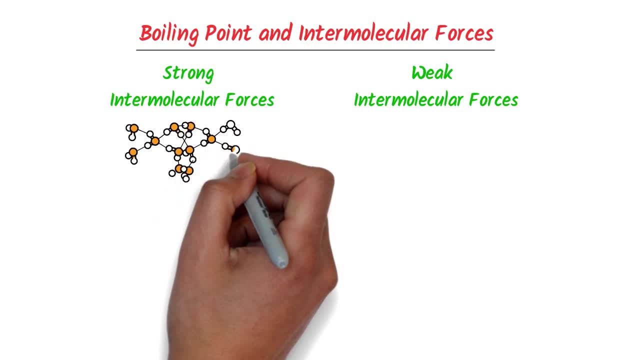 and weak intermolecular forces. You must learn the concept of strong intermolecular forces and weak intermolecular forces. When we cannot easily separate the molecule of a compound, we say that it is a strong intermolecular force. In case of strong intermolecular force, we need more thermal energy to separate the molecule. 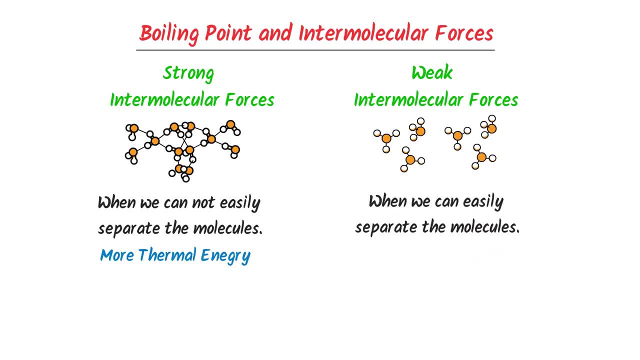 On the other hand, when we can easily separate the molecule of a compound, we say that it is a weak intermolecular force. In case of weak intermolecular force, we need less thermal energy to separate the molecules. In the light of these facts, we say that boiling point is directly proportional to intermolecular. 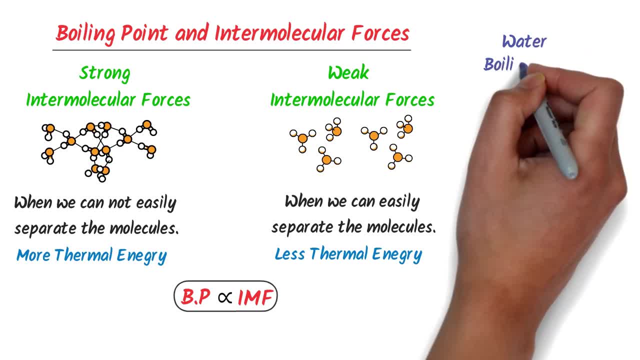 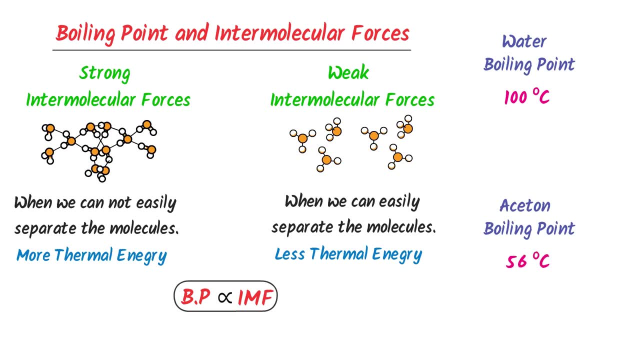 forces. For example, the boiling point of water is 100 degree centigrade and the boiling point of acetone is 50 degree centigrade. Here the boiling point of water is high And the boiling point of acetone is low. 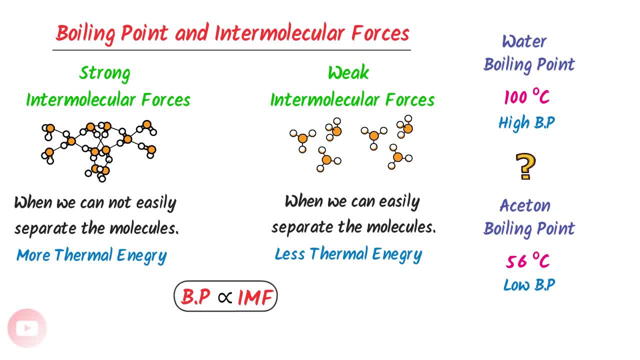 Can you guess that? which compound has strong intermolecular forces? Well, the boiling point of water is high, so it has strong intermolecular forces. On the other hand, the boiling point of acetone is low, so it has weak intermolecular forces. 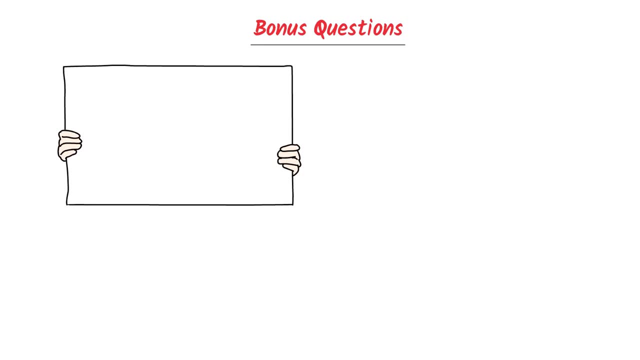 Finally, let me teach you two bonus questions. What is the strongest intermolecular force? Well, the upper water. The answer is hydrogen bonding. Hydrogen bonding occurs when hydrogen is bonded to a strongly electronegative element. For example, consider hydrogen and fluorine. 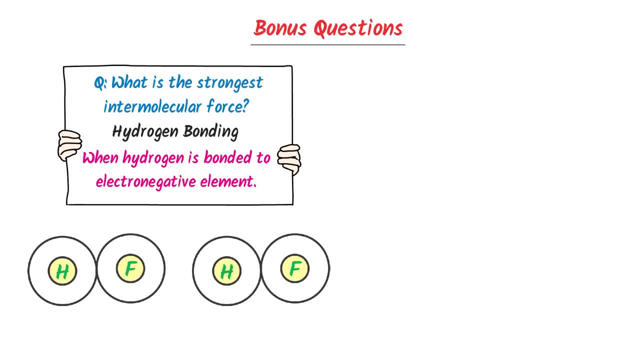 We know that hydrogen has only one electron. therefore it is less negative. One can say that it is almost positive. On the other hand, fluorine atom is highly electronegative atom. This causes very strong attractive force Between weak and strong atoms. 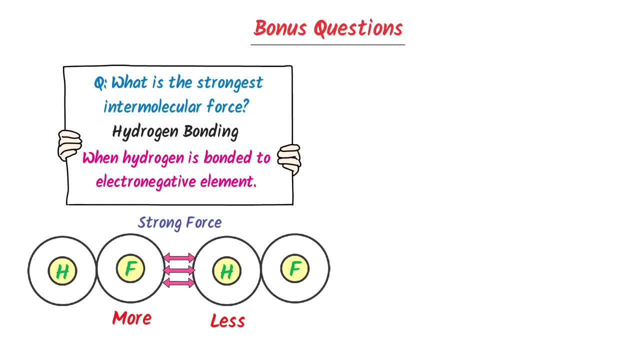 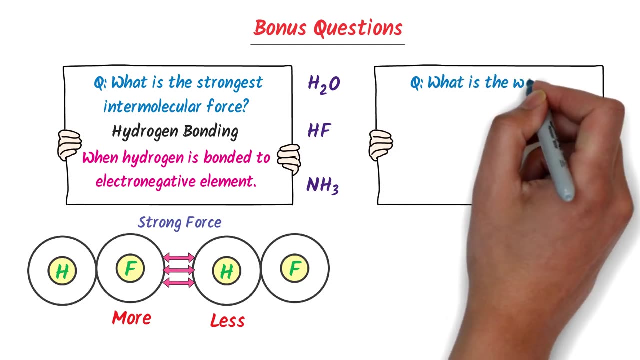 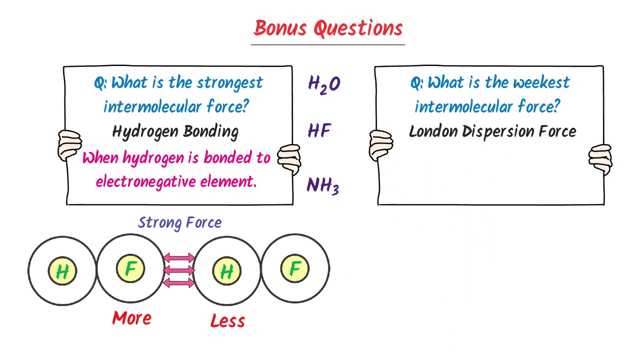 Thus large amount of energy is needed to break this bond. therefore, hydrogen is the strongest intermolecular force. Remember that it exists in hydrogen, fluoride, water and NH3.. Lastly, what is the weakest intermolecular force? Comparatively, we say that London dispersion forces is considered to be the weak intermolecular.